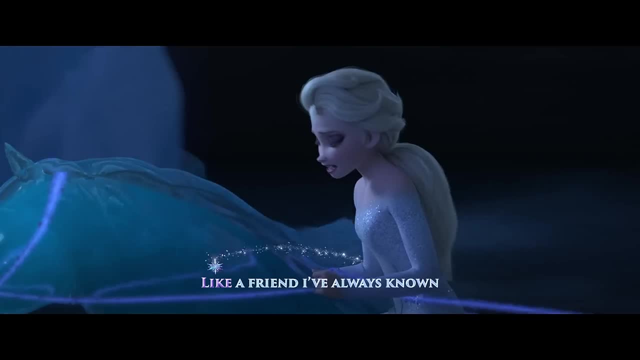 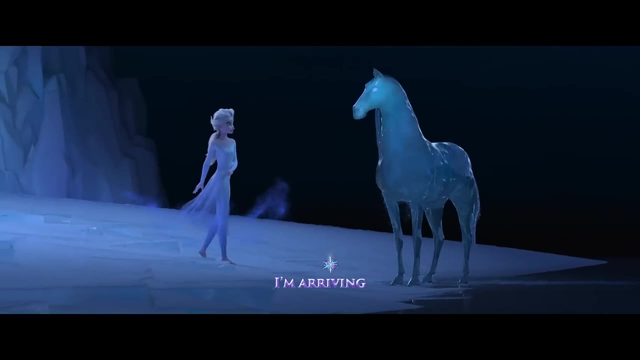 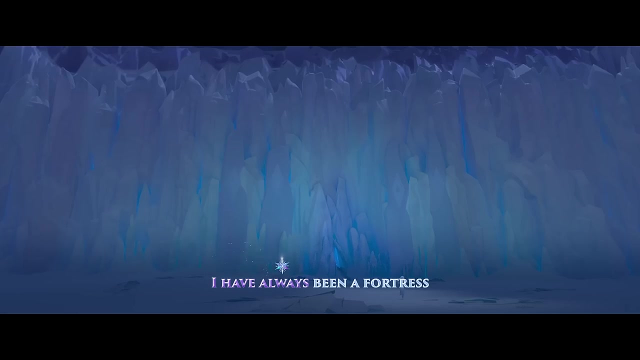 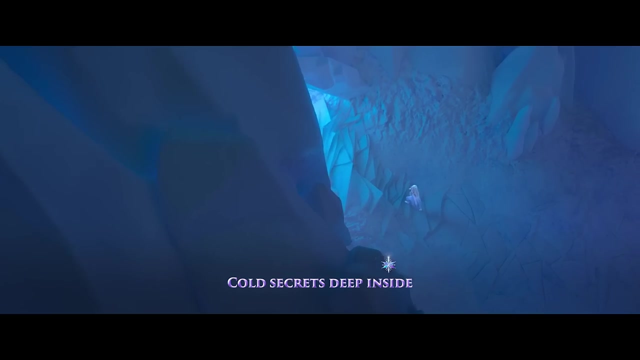 I can sense you there like a friend. I've always known I'm arriving and it feels like I am home. I have always been a fortress cold secrets. deep inside You have secrets too, but you don't have to hide. 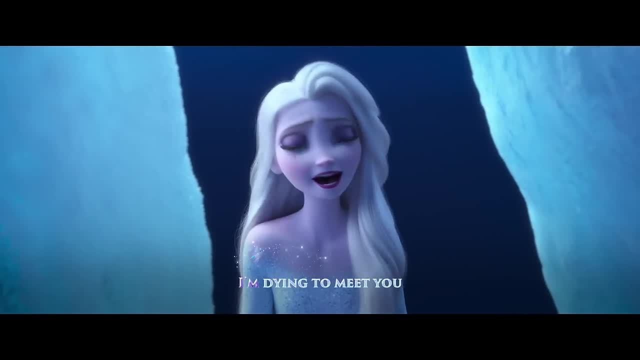 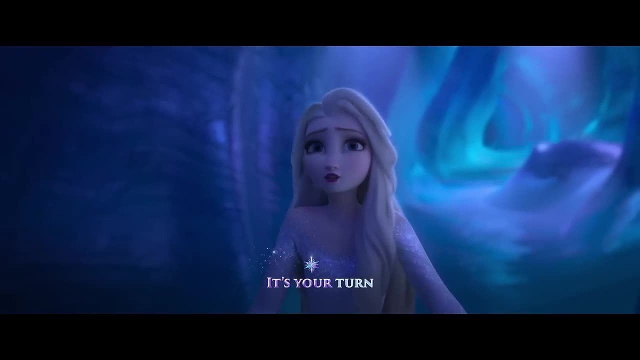 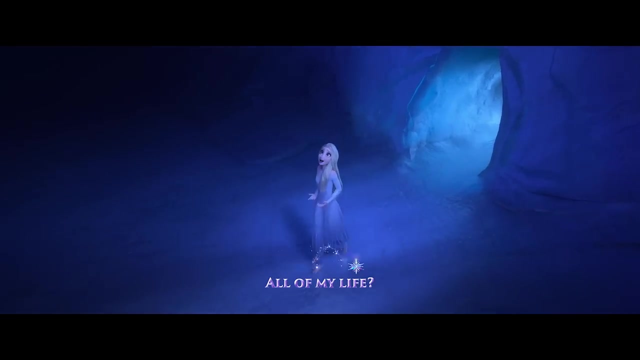 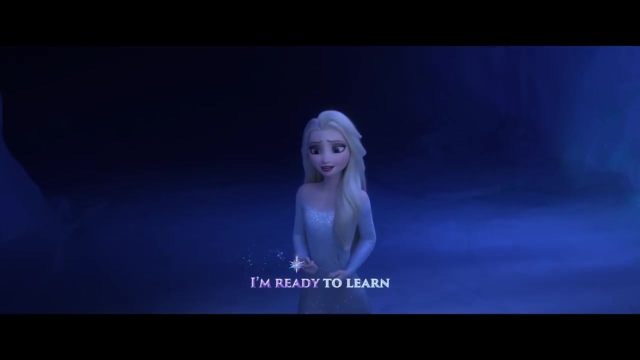 Show yourself, I'm dying to meet you. Show yourself, it's your turn. Are you the one I've been looking for all of my life? Show yourself, I'm ready to learn. Ah-ah-ah-ah-ah-ah-ah-ah. 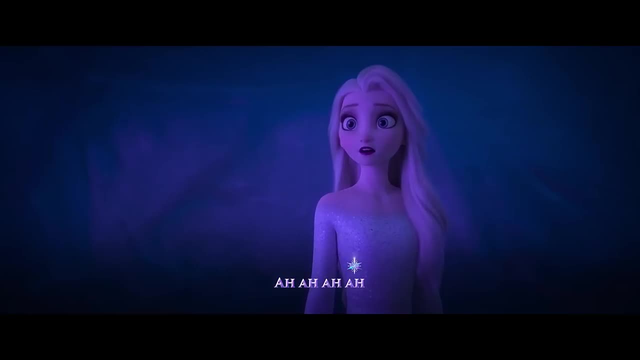 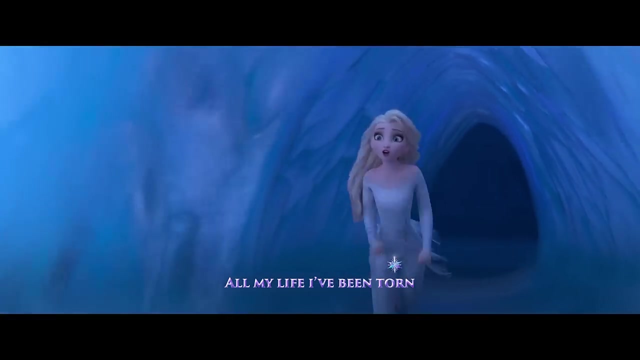 Ah-ah-ah-ah-ah-ah-ah-ah, Ah-ah-ah-ah-ah-ah-ah-ah. I've never felt so certain All my life. I've been torn, But I'm here for a reason. 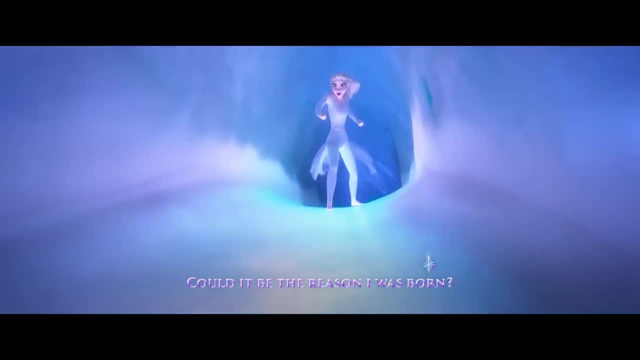 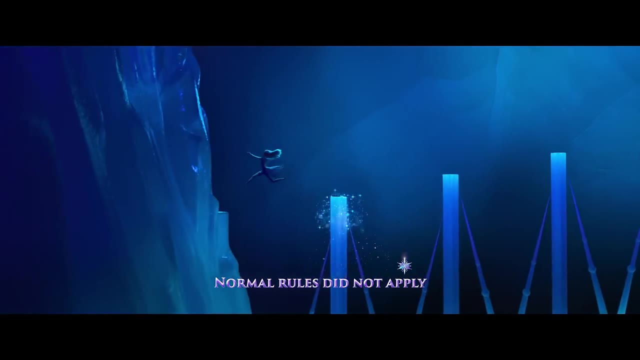 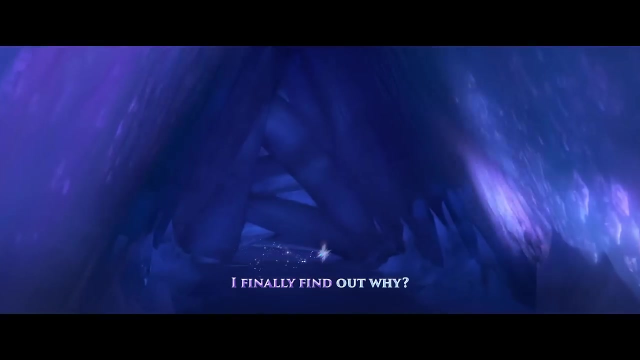 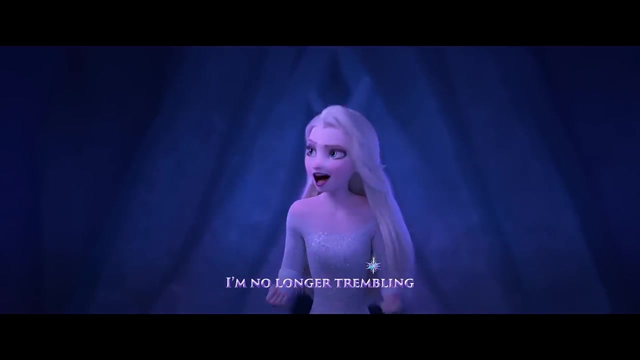 Could it be the reason I was born? I have always been so different. Normal rules did not apply. Is this the day, Are you the way, I finally find out? why? Show yourself. I'm no longer traveling Here I am. I've come so far. 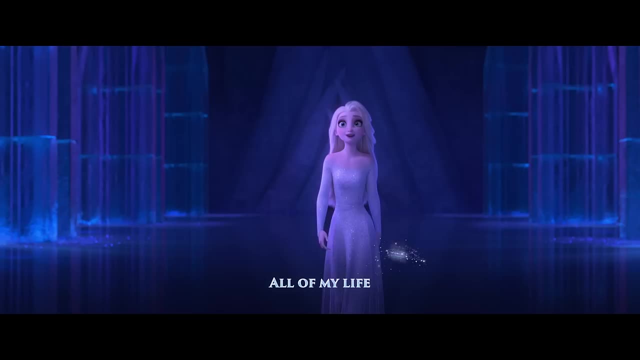 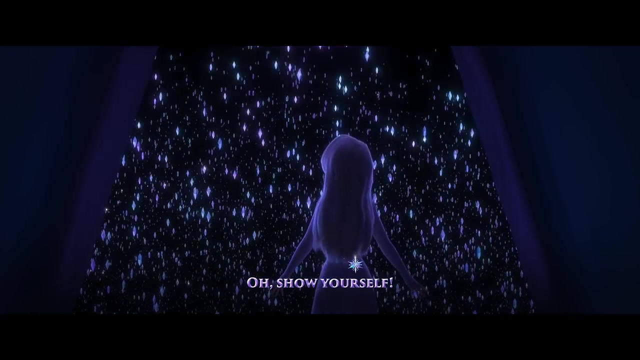 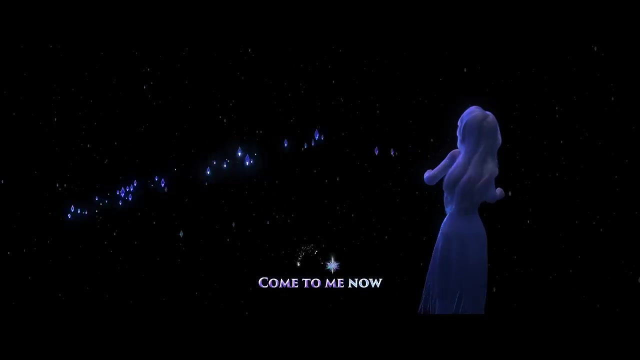 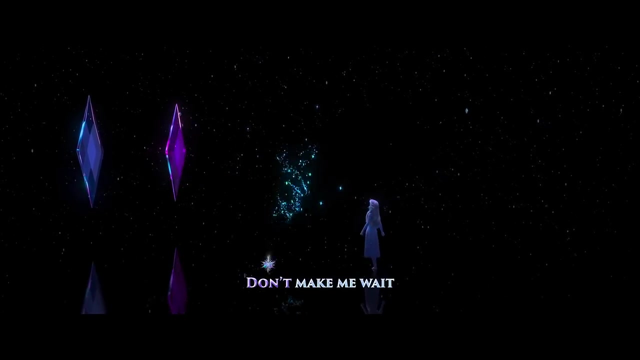 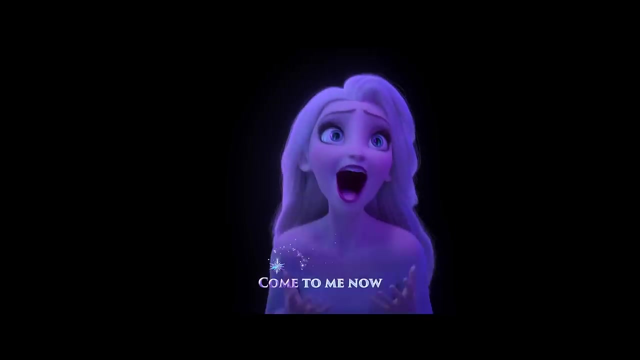 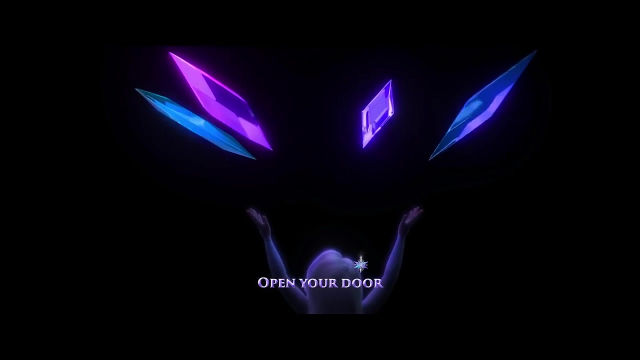 You are the answer I've waited for all of my life. Show yourself, let me see who you are. Come to me now, open your door. Don't make me wait one moment more. Come to me now, open your door. Don't make me wait one moment more.